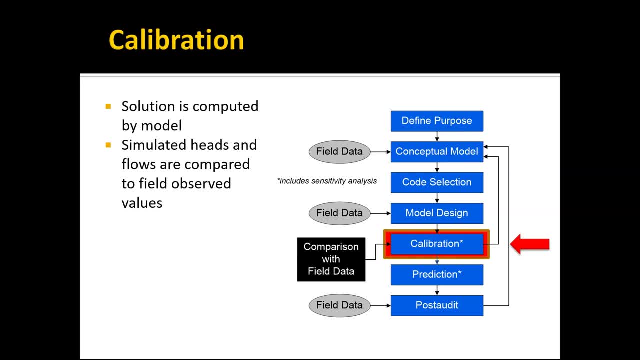 field and invariably they are going to be different. I've never seen a model where first time you run it it gave good results. You always have to do some adjustments. During the model calibration process we iteratively change the input parameters- Hydraulic conductivity, recharge, etc. until the model outputs match your field. 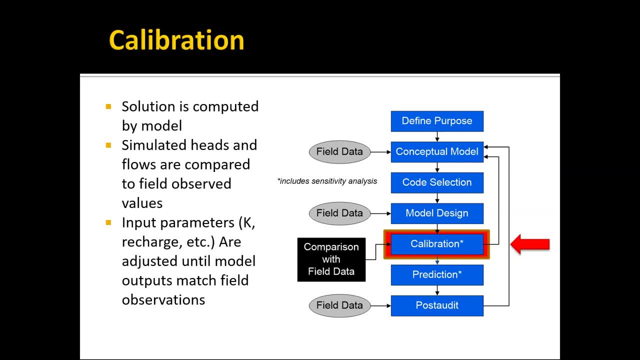 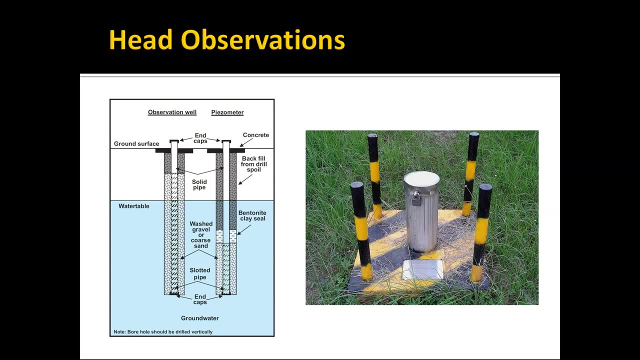 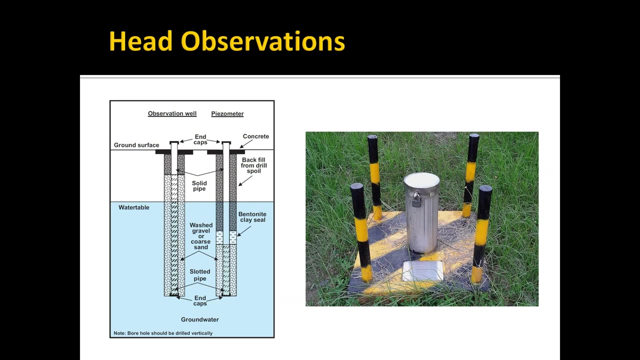 observations. Once you get a good match you're ready to use. you have some confidence in the model and you're ready to use it as a predictive tool. So what are we comparing against? One of the most important parts of this is head observations. These are water table observations that we 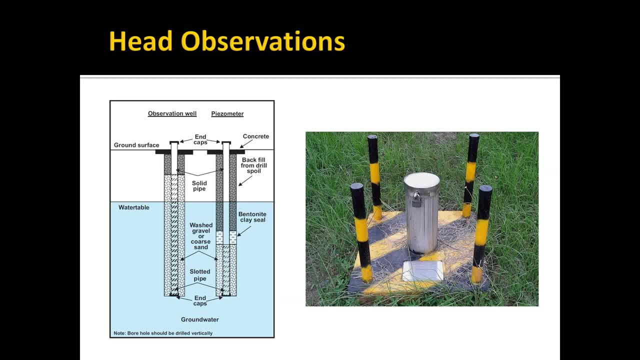 typically collect at observation wells. Hopefully, in the aquifer you're modeling there are a number of monitoring wells. The top of the well looks like the image shown on the right. Those four bars surrounding it are basically there. so if someone drives a lawnmower or some sort of vehicle in, they will damage the 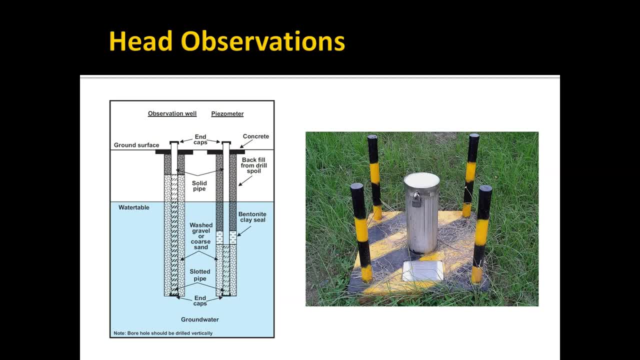 guard posts instead of the actual well which sticks up. So you take the lock off, you drop a tape down into the well and you measure the depth down to the water table and then record that and that becomes a very valuable observation On the left. as you will see, this is kind of what the typical schematic of the construction. 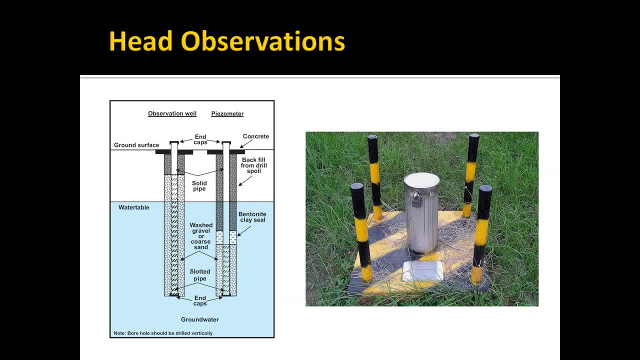 of the monitor. well, You have a pipe in the middle, at the bottom, at some point there's a screened interval where the water is allowed to flow into the pipe. between that pipe and the top, that's called the riser, and around the slotted part of the pipe you have gravel or some coarse material that. 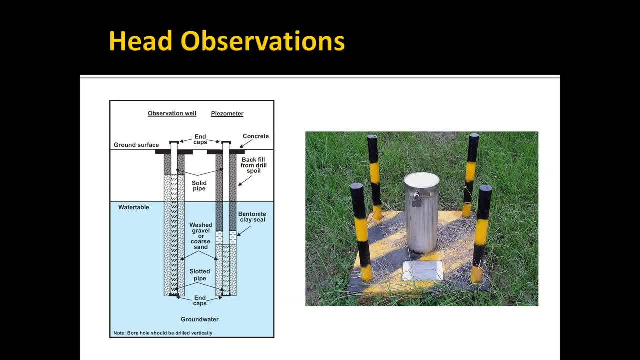 the water can flow through freely. and then there are two kind of approaches here. the one on the left has a really long slotted screen and the one on the right the there the slotted screen is isolated down deeper into the aquifer and then it's sealed. but the water flows into the pipe and then they both. 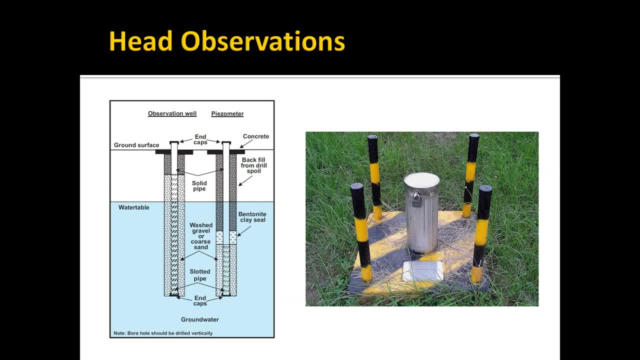 effectively measure the same water level, the one on the right we typically refer to as a piezometer. just you know that, having an isolated opening and and then you know, measuring how far the water rises in the pipe. we typically call that a piezometer, but those terms are sometimes used in 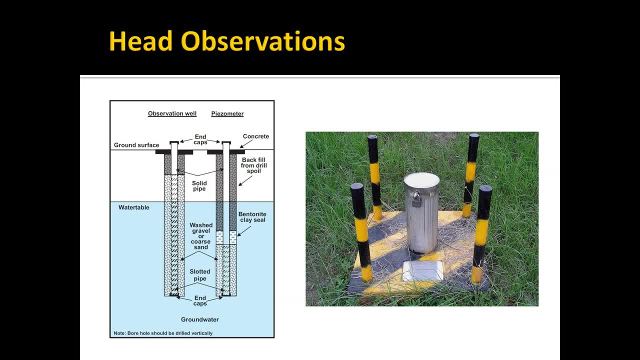 the aquifer interchangeably. I should also mention that sometimes we do measurements in production wells. so you have a well that's pumping, you turn it off or you turn it off and then you measure the water level. the problem with that is when you pump a well it causes a cone of depression where the water table is. lowered due to the pumping and then when you turn it off, it takes. if it's a highly porous aquifer, it's not going to be able to pump the water out of the aquifer. it will rebound fairly quickly, even you know, in a matter of minutes or hours. 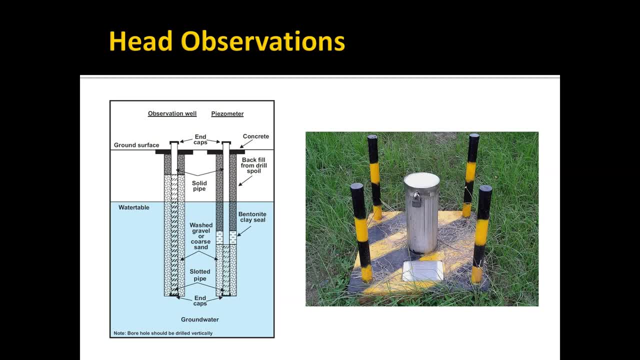 but if it's a lower permeability aquifer, it may take several days for that to rebound. for that reason, a lot of times wells are measured in the winter, when they're not pumping, if they're agricultural wells, and so you always have to be careful of that effect and be a little bit careful when you use water. 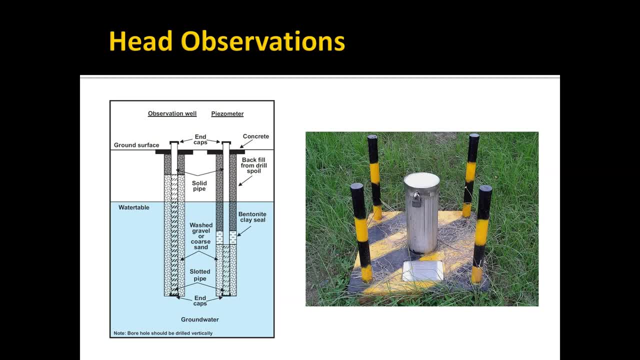 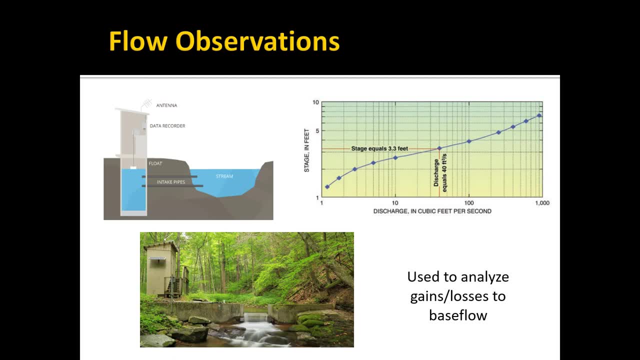 levels obtained from production wells. another type of very important observation is a flow observation and this is basically the how much water is flowing in a stream and specifically what we want to know, what you need to have these measurements in pairs, normally, because you need to know how much the flow has changed. 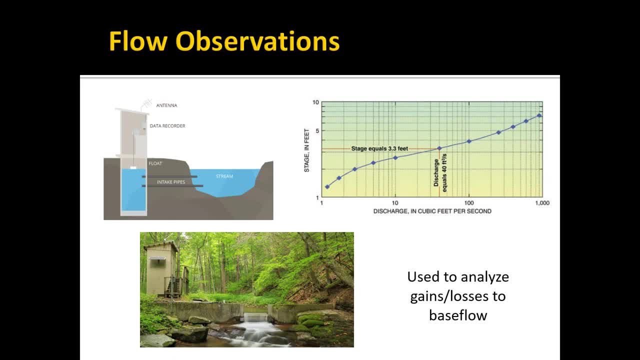 between two points on a stream, because that represents either a gain or a loss from groundwater. now, of course, you measure this in periods when there's not a big precipitation event and in some cases you can get away with, if you have a stream that that that starts flowing in the aquifer. 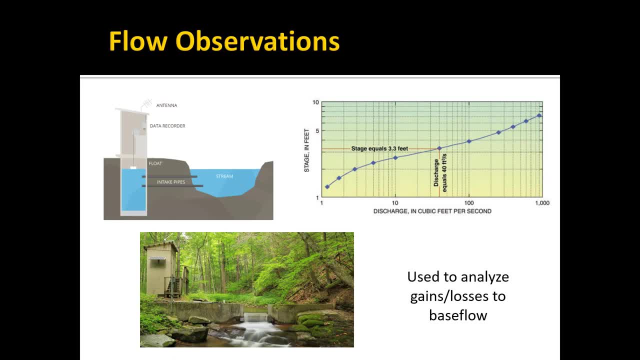 and you have a single measurement down downstream and you measure it during a non-precipitation event or under base flow conditions, then you can get away with the single streamflow measurement. but again, the idea is we want to measure how much of the base flow is coming from. is it the gaining or losing stream? and 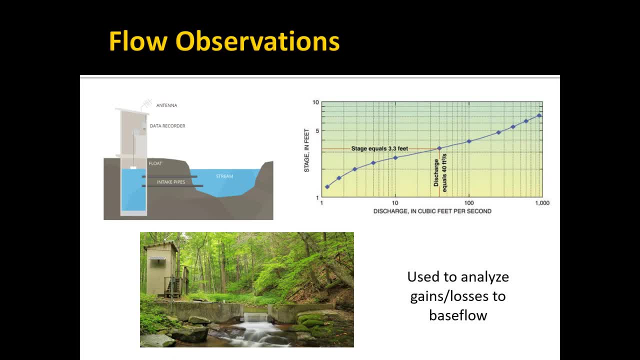 what is? what is the quantity of that gain or loss? that's something that use. use that value to measure water- waterочь個- when we calibrate our groundwater model. So if we have a groundwater model and we're using, say, the river package, 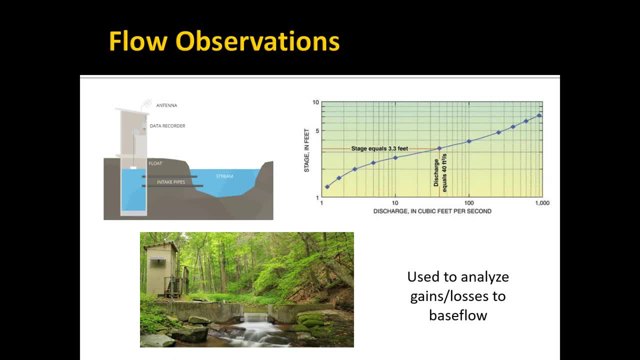 or the drain package or something. part of the output from the model is how much water is going into the stream or going from the stream to the aquifer, and that should match reasonably close with what you observe in the field. There are a couple ways we measure, or there are a number of ways we measure, stream flow. 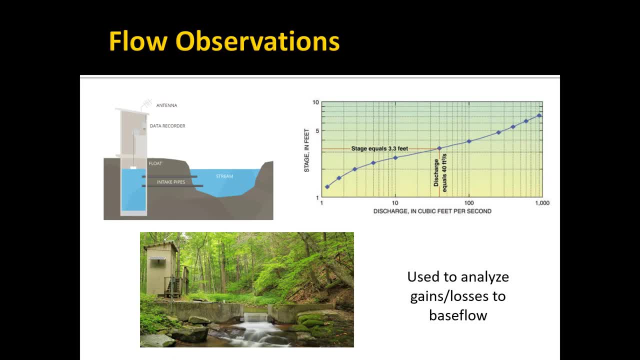 So the top diagram on the left. it's measuring basically the stage in the river and presumably someone has gone in and measured as the stream has flowed at different stages. they measure the velocity across the stream and then from that there's a way to calculate. 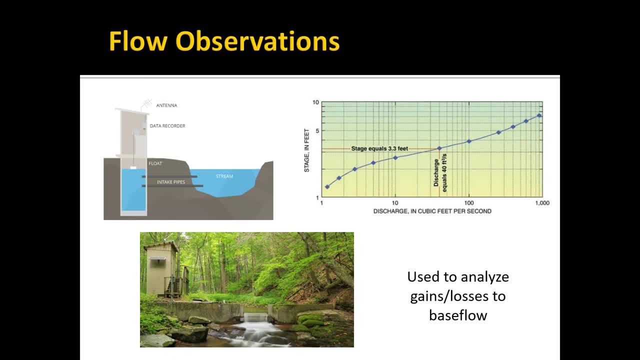 how much stream flow is going to flow across the stream And if you do that at a number of different stages, or a stage again is the elevation of the water in the stream, and for each of these stages you measure the discharge. 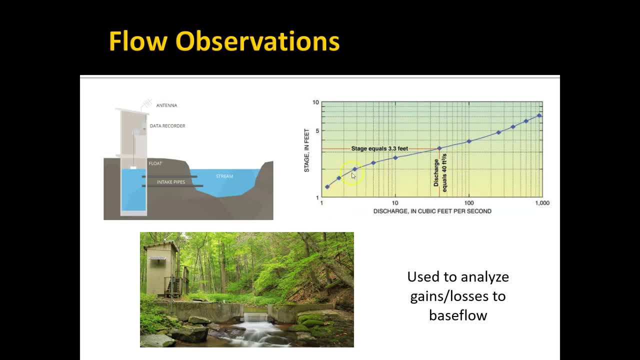 So, on the diagram over on the right, each of these dots could represent a point in time where someone has measured the stage and then, using a velocity meter, calculated how fast the water is flowing through the different stages. So you can see how fast the water is flowing through the different stages of the stream. 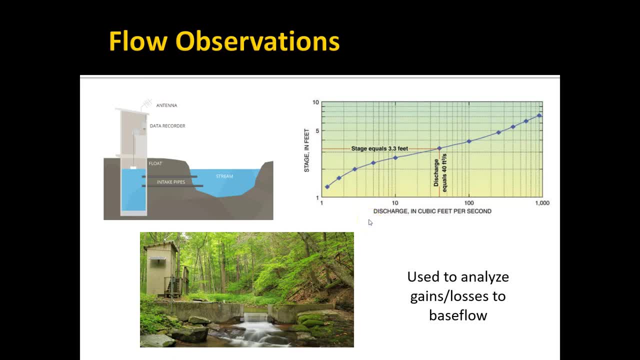 and from that estimated discharge. Once you've done that, you come up with a stage discharge curve and from that point, if you measure the stage, you can just scale off what the discharge is, and so you can have a real-time measurement of the stage in the stream. 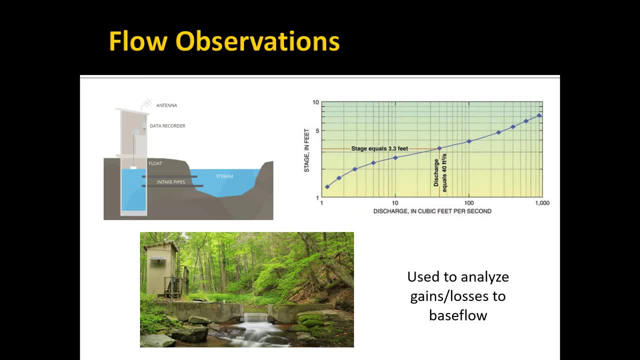 In the United States, the United States Geologic Survey has instrumented a lot of data, a large number of streams around the country, and a lot of these have telemetry, where they record the stage and then transmit it electronically from a recording station to the USGS. 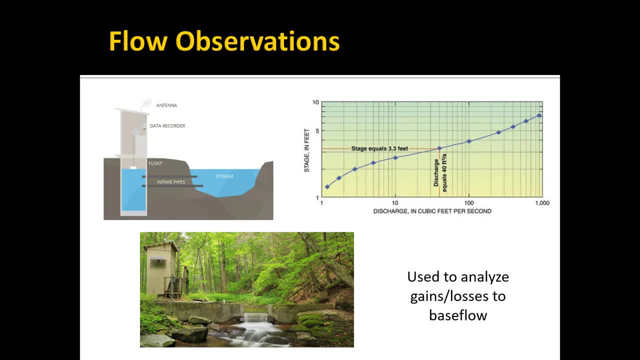 which then they publish these through web services or on a website In the lower left. this is a weir For small streams. sometimes we build these channels that the water goes through, where we can even more accurately determine the flow rate based on the elevation of the water. 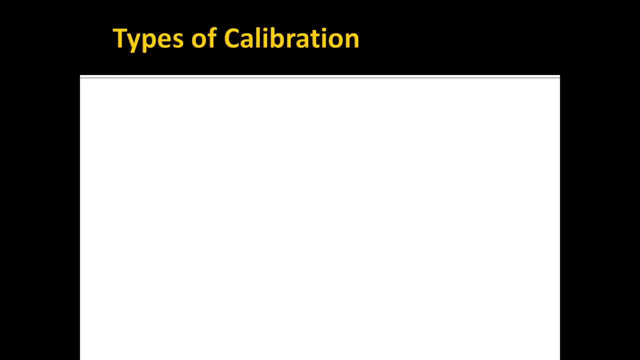 And so that's another very important type of observation. So again, so calibration is changing the model inputs until the outputs match the heads and flows you've observed in the field. There are two basic types of calibration. One is just trial and error, which means we look at the model. 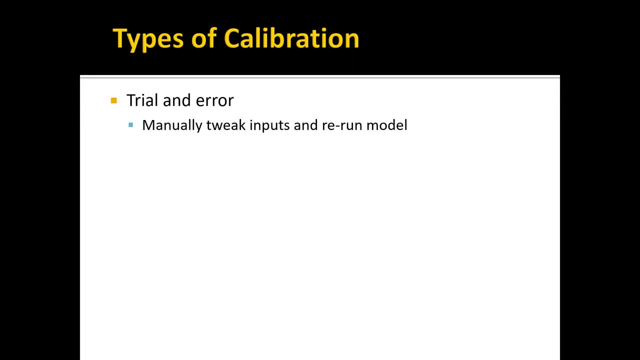 We say, well, my heads are too high, Maybe I need to reduce recharge. So you reduce your recharge and run the model again. Maybe the next round you change the hydraulic conductivity. And a pretty simple and straightforward way to calibrate your model. 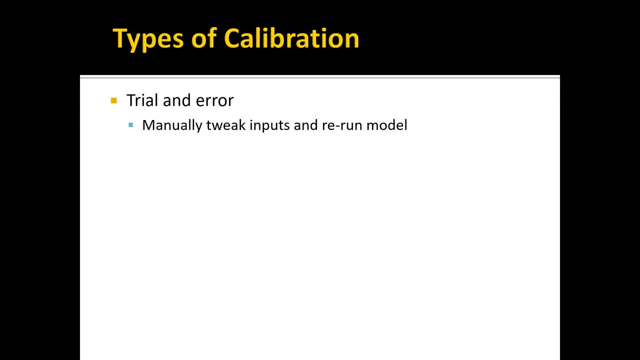 You know you should always start with trial and error, or we sometimes would call this manual calibration. Okay, And I've seen people who are really good at manual calibration and they can fine-tune a model just through hard work and they can do it fairly quickly. 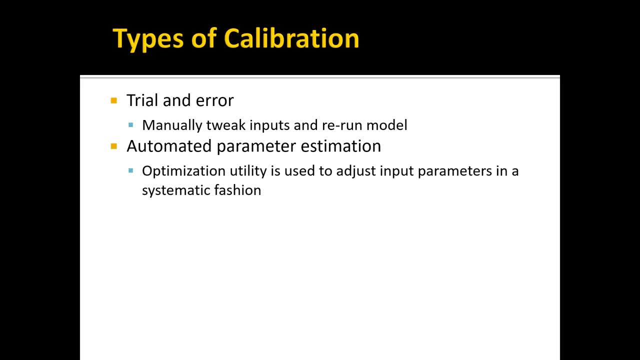 Another type is called automated parameter estimation And basically what we do is you use an optimization tool and you tell it what parts of the model inputs you want it to change, and then it takes over control of your model and automatically runs the model tens, hundreds, even thousands of times. 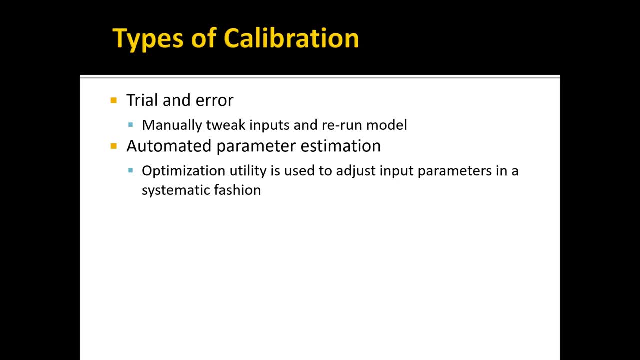 and systematically changes the inputs and then measures. it looks at the output from the model, compares that to the field observations, and it continues Until the difference, the overall difference, between the model simulated values and the field observed values is minimized. And there have been a number of utilities like this over the years that come and go. 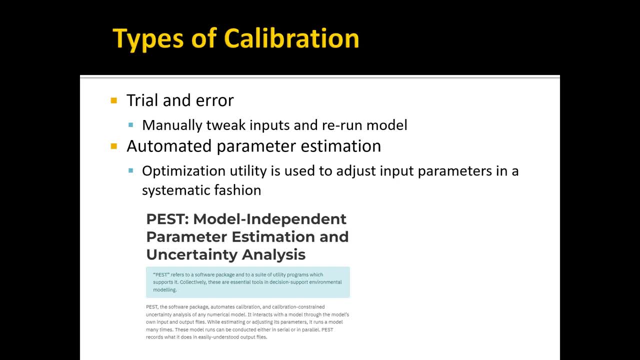 but there's one that's kind of stuck around and become the dominant model, and that is a utility called PEST, which stands for parameter estimation, And this is a product, Okay, You can download off the web. It comes packaged with GMS and we will be using PEST quite extensively. 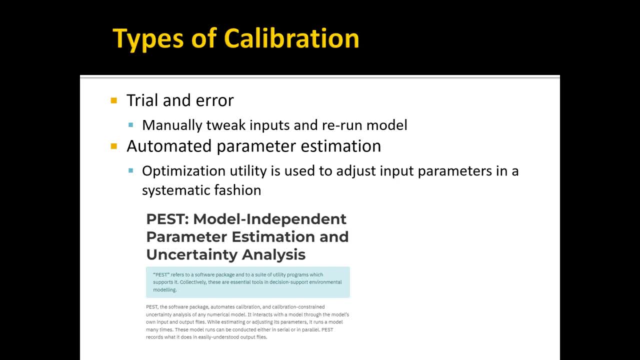 It was originally developed by John Doherty from Brisbane, Australia, a good friend of mine, a great guy, and it's a really powerful tool to help you calibrate your model. You're going to come to really appreciate it once you try it. 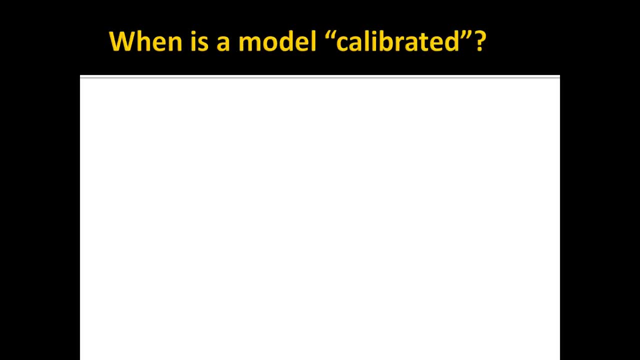 So how do we tell when a model is calibrated? First of all, we should never expect a perfect fit between our simulated and observed values. It's just unrealistic for a number of reasons. First of all, measurement error. Measuring the water levels is not an exact process. 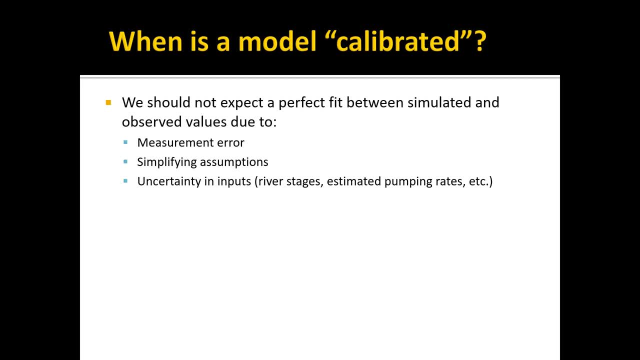 Maybe you're measuring in a well that's a production well and the water levels haven't fully rebounded. Once you measure the depth of the water table, you have to convert that to a water table elevation. To do that, you need to know the elevation of the top of the well. 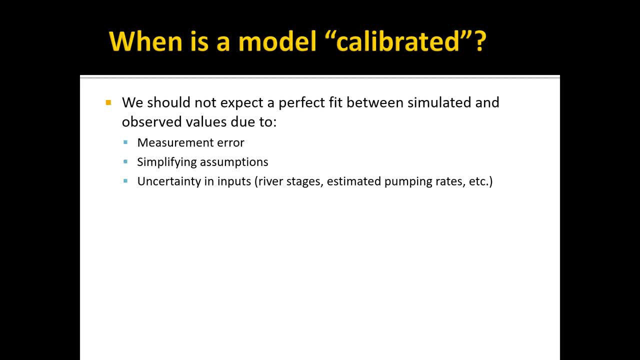 Sometimes we survey that. Sometimes we just guess it based on looking at a contour map. Well, that's going to have significant error built in. So there are a number of opportunities for measurement error to creep in. Also, your model is not reality. 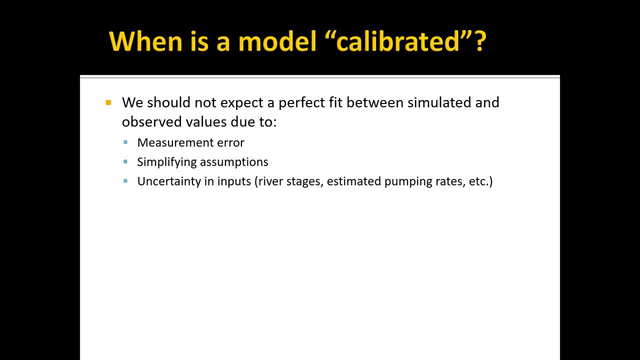 It's a simplified version of reality And therefore we should never expect it to perfectly reproduce what's happening. And then, of course, there's a lot of uncertainty on our inputs. Maybe the pumping rates we're using are not really the actual pumping rates. 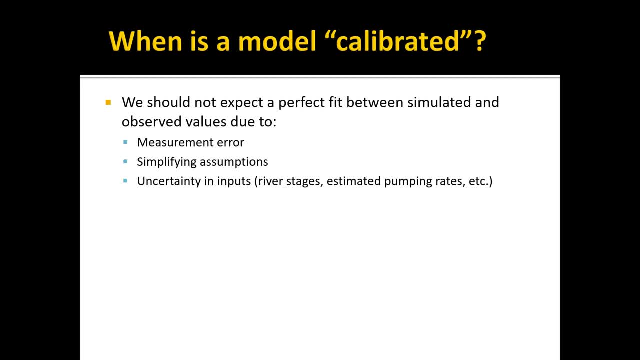 that have happened over time Could be the river stages are wrong. Maybe we've made some poor assumptions. We've made some poor assumptions on certain parts of our inputs. Because of that, we shouldn't expect a perfect fit, But what we generally try to do is get the simulated values. 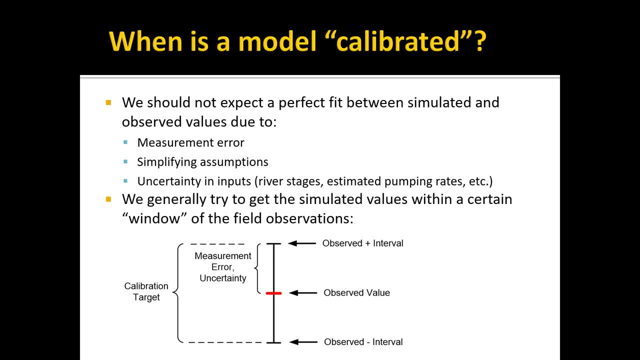 just within some window of the field observations. One way to look at this is, if you have an observed value, you can come up with something We call that a calibration target. You decide on an interval which can be a function of the measurement error or uncertainty. 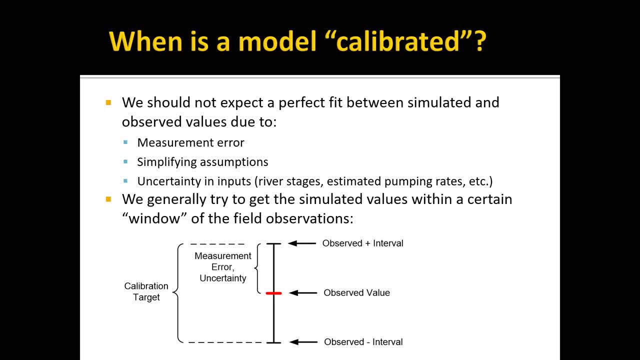 or just general judgment. Maybe you say, well, we're hoping to get the heads within five meters or three meters or something of the observed values And that can help guide the process and help you decide when you're getting close, But ultimately you just keep minimizing the error. 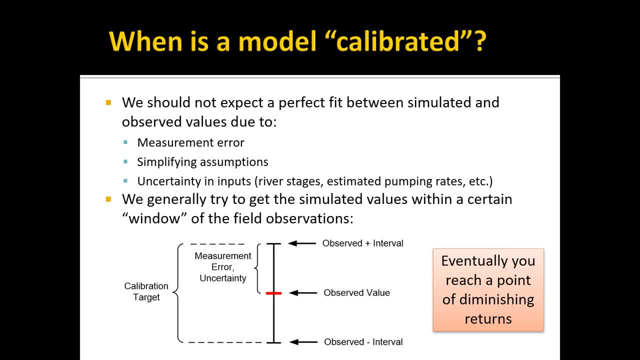 And the error is defined as the difference between the computed and observed values. Until you reach a point of diminishing returns, you're going to get to a point where any change you make to the model makes things worse and not better, And at that point you can reasonably say that it's calibrated the best. 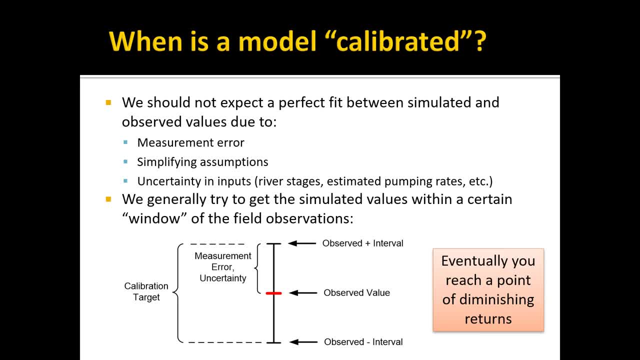 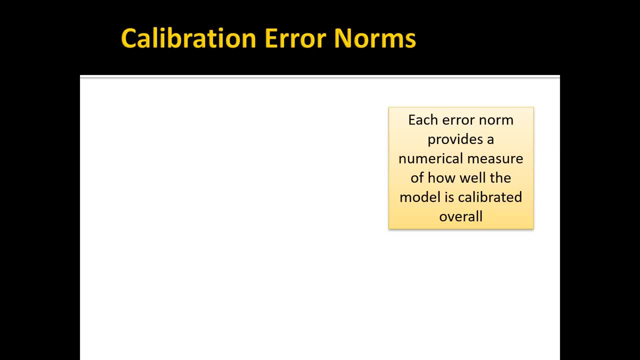 that you can expect under the circumstances, But a lot of this comes just through judgment. So when we're looking at overall calibrations, we're going to look at the values. So what we're going to look at is the total error. 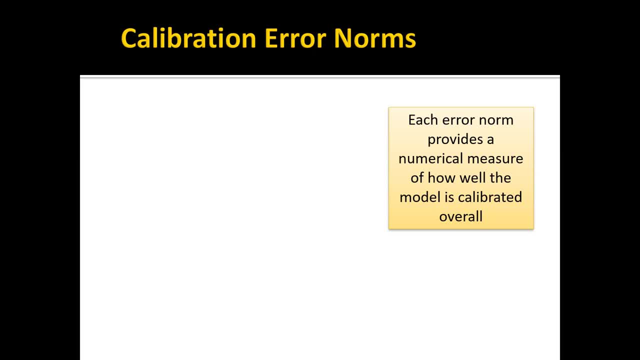 And we're going to look at the total error in the calibration It's customary to have some global error norm. An error norm is a numerical measure of how well the model is calibrated overall, So not at an individual point, but over the whole model. what is the total error? 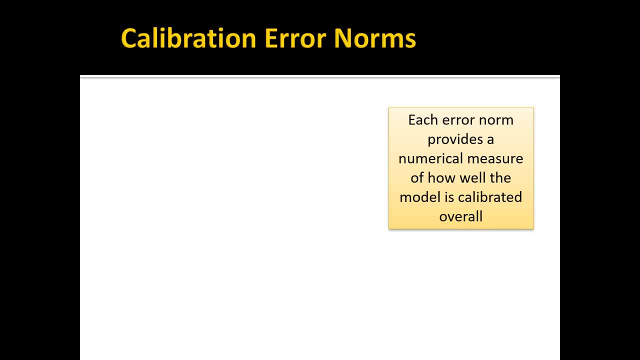 And there are a number of ways that you can do this, And we typically look at a number of different measures. The simplest one is the mean error, And the mean error can be an error. that can be a complete error, And we typically look at a number of different measures. 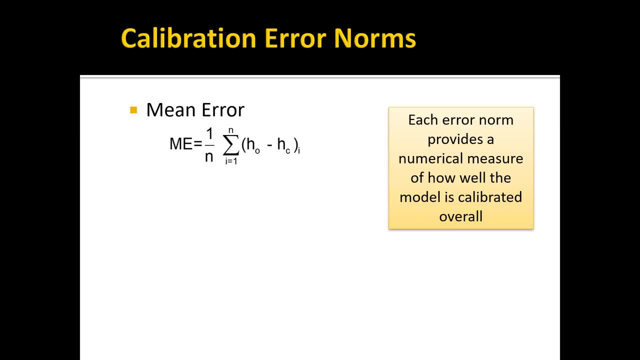 The simplest one is the mean error. these equations are written in terms of heads. you could do the same thing with flows. so if we look at an individual monitoring, well, and we look at the difference between the observed head and the computed head, HO minus HC, that is. 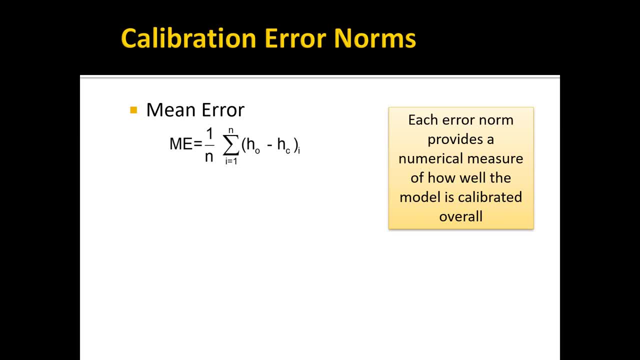 what we call the residual and if you add those up and divide by the total number of observations, you have that mean error or the average error. so you know this can be positive or negative. let's say it's negative. two point five meters, that means on average your heads are two and a half meters. let's see HC. that means 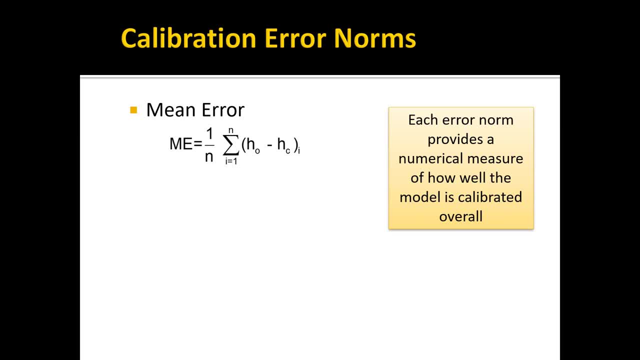 that your observed values are two and a half meters below the computed values and you need to bring your computed values down. and so this is- this should be a pretty simple and intuitive error norm. you now, if you look at this, it's theoretically possible that you could. 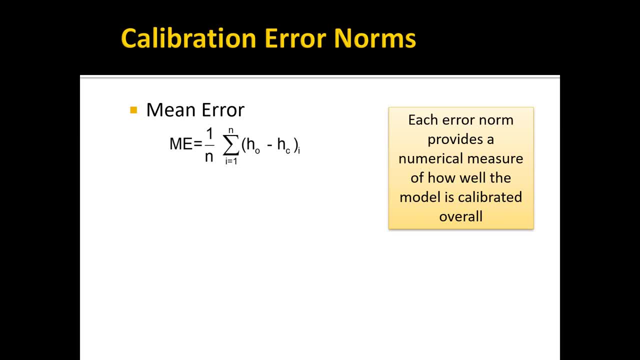 have a mean error that's near zero, but there still could be quite a bit of error at individual wells, and so another measure is called the mean absolute error. in this case we take the individual residuals and we take the absolute value of each of those, and then we take the average of that. so for 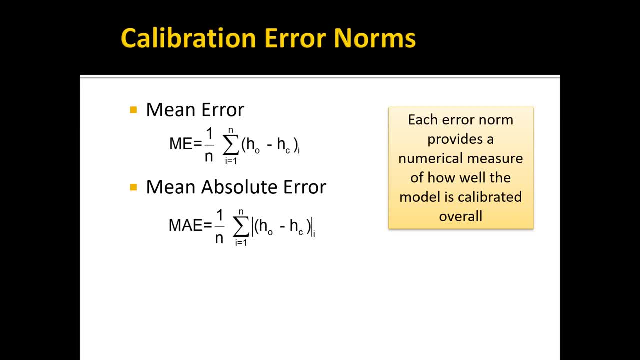 average of that. we take the absolute value of each of those and then we take the average of that. so, for example, if I did this process and then I got a mean absolute error of three point one meters, that would mean that you know whether it's too high or too low the mean. 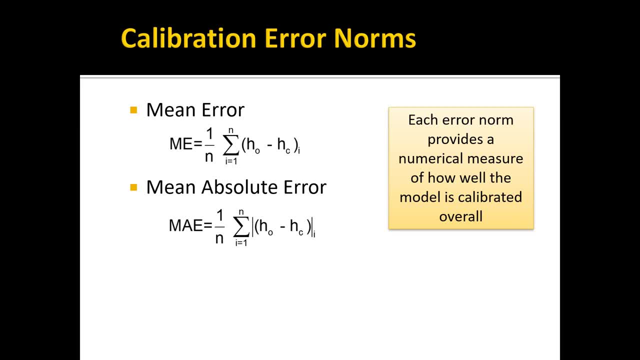 residual magnitude is about 3.1 meters, and so generally we use these two in combination. the me: we want to see the mean error around zero. that shows that your errors are balanced between positive and negative errors. then you want, you just want- to minimize the mean absolute error. then there's 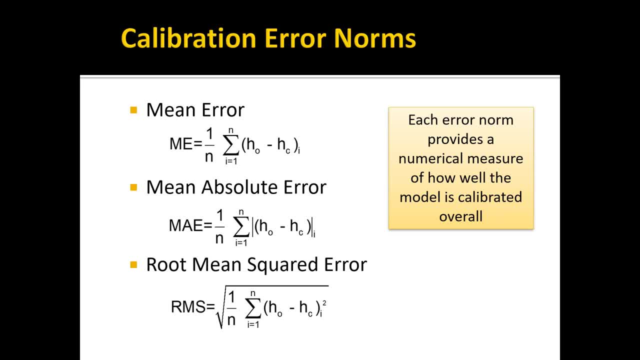 another one called the root mean squared error. this is similar to the mean absolute error: instead of taking the absolute value, we square the residuals and again that makes everything positive. and then we take the average of those squared residuals and then take the square root of that. it's just another. 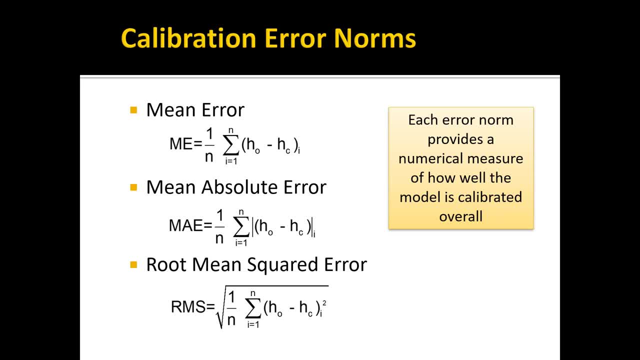 way of doing a mean. it is again, as is the case of the mean absolute error. it tells you about the magnitude of your error. one difference between the RMS, or root mean, squared error, and then, and the mean absolute error, is if you have a few large outliers. 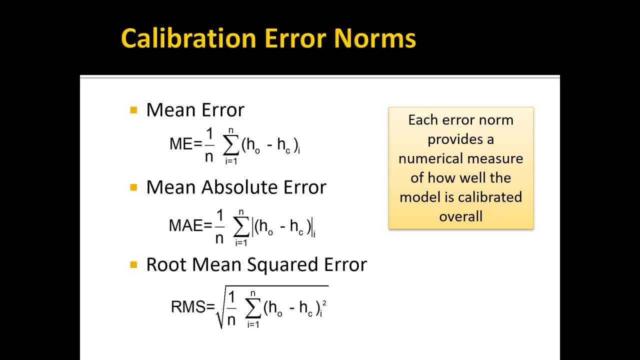 that have a large residual. those will really be magnified with the root mean squared error. and so if your root mean squared error is is significantly larger than your mean absolute error, then it means your errors are. you know you have a number of outliers or large deviations that you need to be concerned with. so 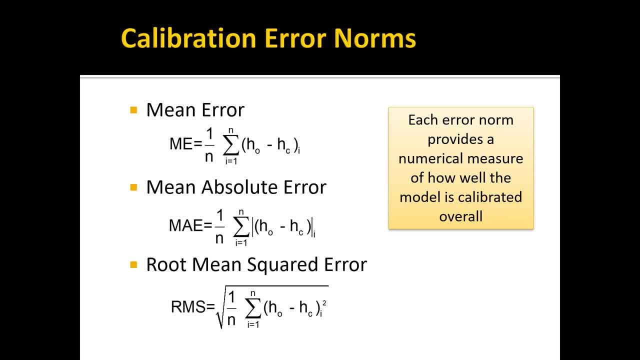 each of these have play an important role in GMS are reported and it's generally good idea to look at. look at all three of these now. another thing that we do sometimes is you take these same equations and you can apply a weight to individual observations. the weight in 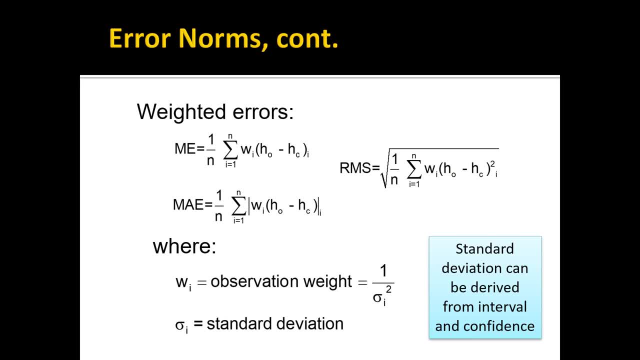 many cases we just assume a uniform weight. we weight all of our observations equally to move the weight of the data from one single observation to another, more or less evenly to all three observations. so we can make a lot of changes to a product every time we take a look at our data. this will allow us to 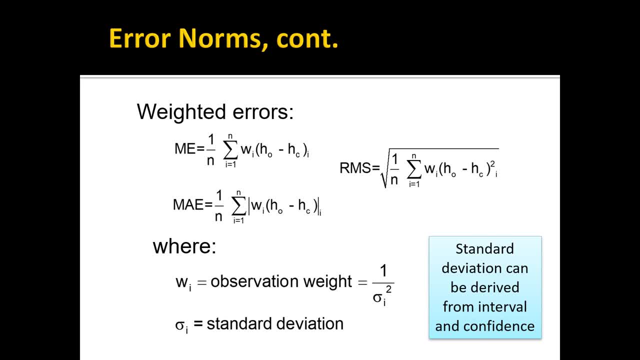 take a look at this product every time we take a look at our data. this will allow us to, But this allows you to give greater emphasis on certain observations And if you want to look at this, one way to look at this is the weight can be defined. 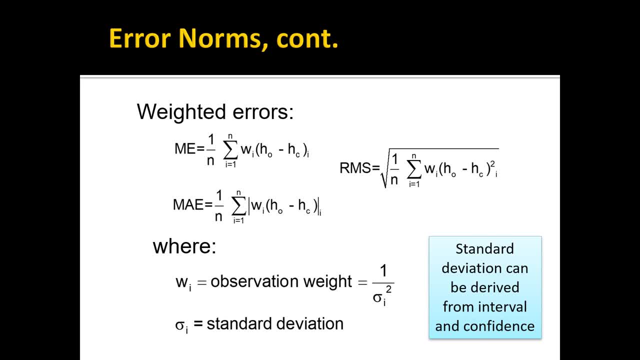 as 1 over the standard deviation, squared where the standard deviation is the standard deviation of the measurement errors for the observation. So if you had some way to determine over time what the typical error is in the observation and could get a normal distribution of that and a standard deviation, that would be a 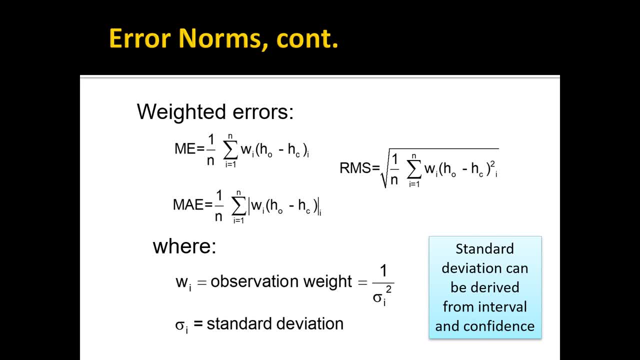 way to come up with your observation weight. You can also, if you assume a normal distribution, you can define an interval and a confidence. So an interval and confidence, for example, could be The interval, could be your calibration target. So you say: well, I think it's. 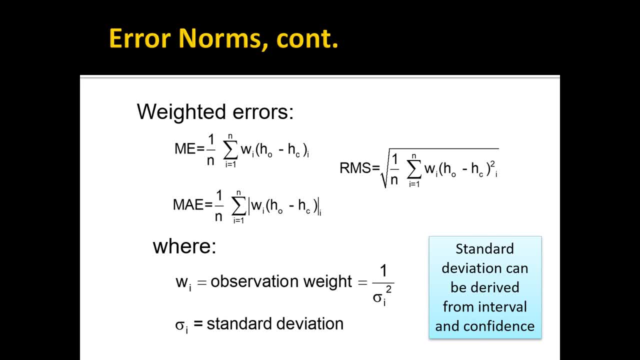 Have 95% confidence that the errors are within 2 meters, Then from that 2 meter and 95% value you can come up with a standard deviation and then convert that to an observation weight And there's a way to automate that in GMS. 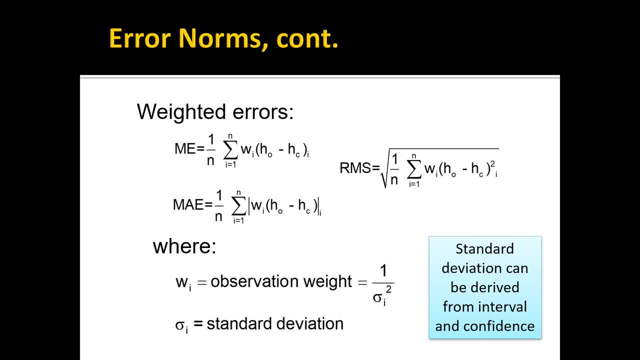 But if you assume the same confidence, Confidence interval, then if you just give each well a different interval, your calibration target, maybe some of them you say it's 1 meter, others 2, others 3,, others 5, the ones. 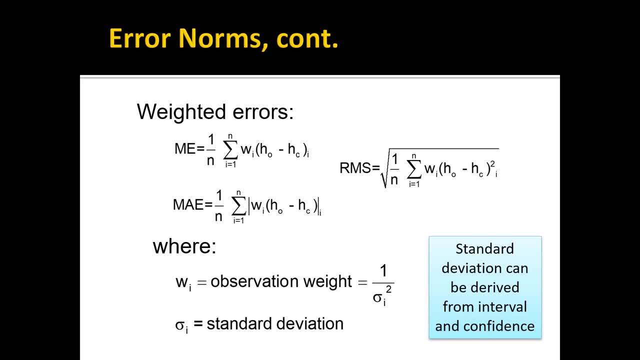 with the larger interval or target are going to have a smaller weight, because the bigger the weight, the bigger the interval, the bigger the standard deviation. And that's kind of intuitive. If I have an observation where I want to get it within 1 meter, then that's going to have. 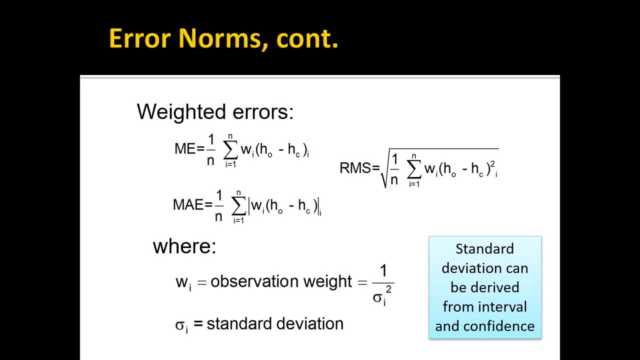 a higher weight than if I have another one, where I'm okay if it's anywhere within 5 meters. So that's one way to look at this. But in general, like I say, in most cases we assign the weights evenly, But you can have different weights for different observations if you like. 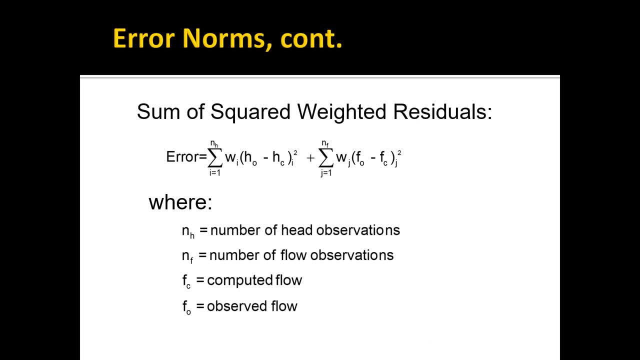 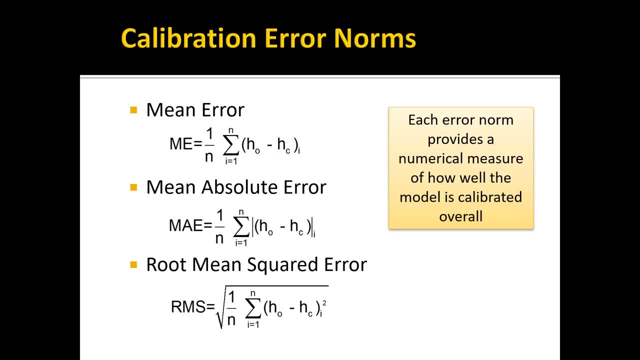 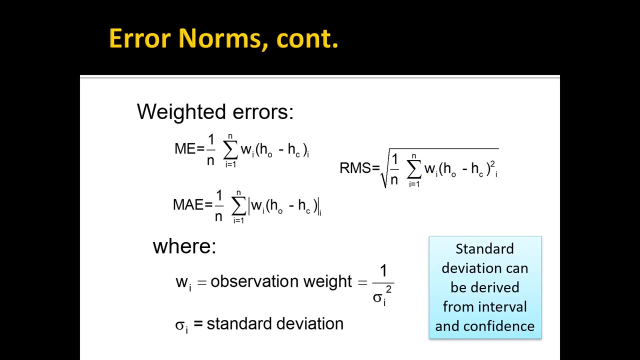 Finally, there is a single error norm that includes both heads and flows, Both of these weighted and unweighted equations that I showed you. these are written in terms of heads, But if you substitute flow, the F for the H there and you use gains and losses in streams, 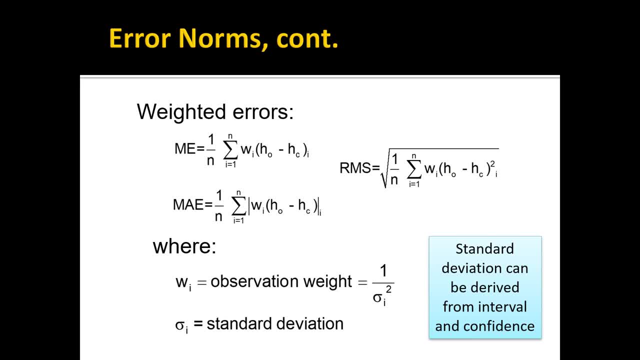 you can come up with the same weight. But you'd have a ME, MAE and all sorts of different weights. But if you substitute the F for the H there and you use gains and losses in streams, you can come up with the same weight. 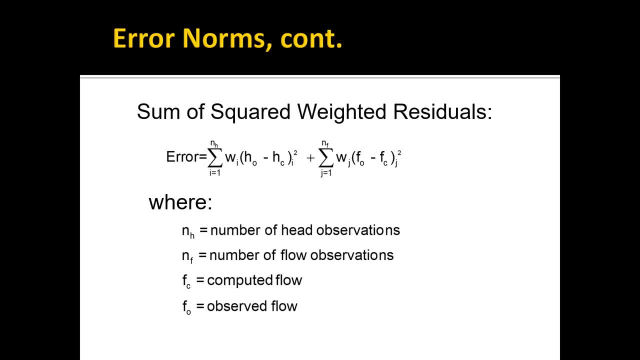 And if you combine both heads and flows- the F for the H there- and you use gains and losses in streams, you can come up with the same weight. This equation is to combine both your heads and flows into a single error value. It's the sum of the squared weighted residuals. 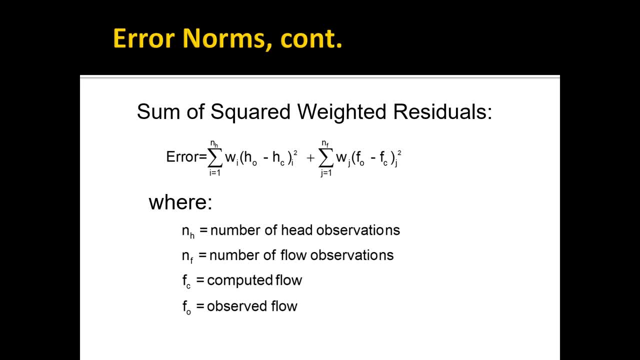 You take the head differences squared and the flow differences squared, You give each of them weight And add them. We do it like this, but that should do it for the next two Almost 50 Description and, subtracting from it Five, 50.. 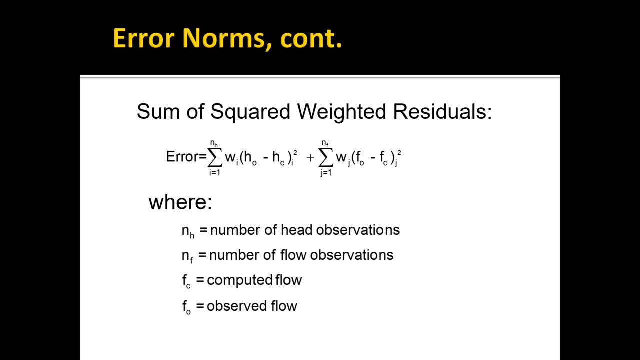 Water, 살�ling and one flow rate. add them up, it's just a song. it's not an average, it's a song and the number by itself is not. that doesn't tell you that much. but what what you want to know on this is is how that number is changing as you calibrate your model, so as you. 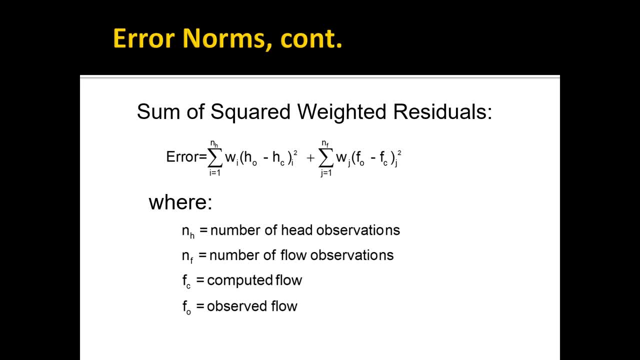 try changing your hydraulic conductivity, your recharge or conductance and so forth. if you look at the sum of squared weighted residuals, that number should be going down. so when you use a parameter estimation utility like pest, this is the single error norm that it looks at, because it does combine both heads and 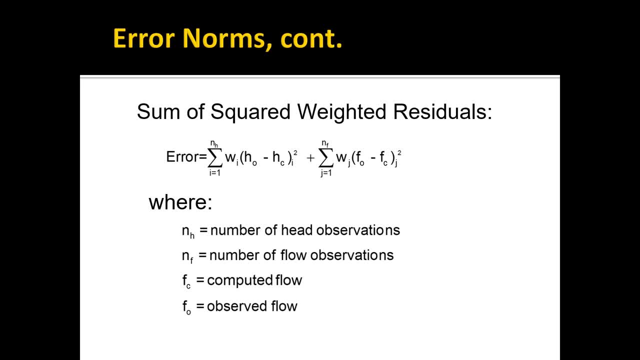 flows. now, something that's really important here: if you're combining heads, the units are length. flows, the units are length cubed per time. so it's kind of weird that you're combining, you know, two different sets of units into a single value, but again it's just used. 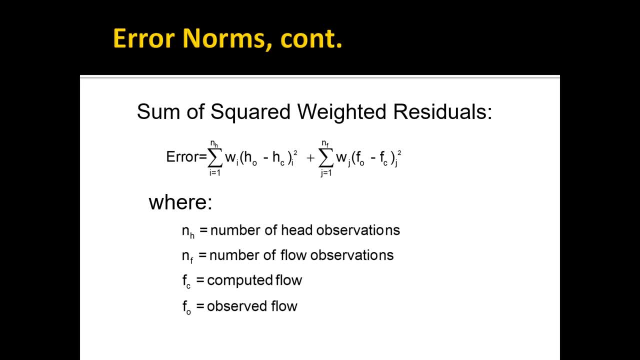 for to determine relative differences. but in order for this to work well, you have to ensure that you have good weights. so the weights for the heads: again, we get that from the interval if you, as long as you, use a reasonable interval on your calibration target, you know one to five to ten meters, something. 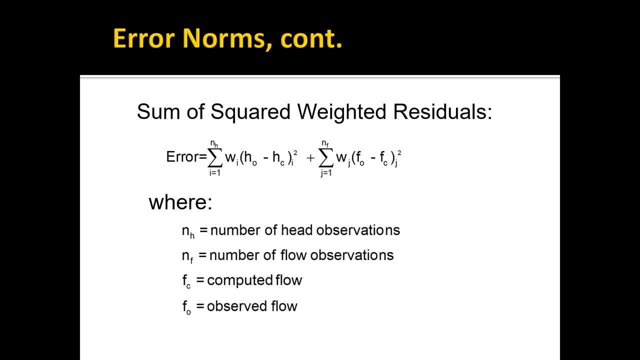 like that. it works out fine. and then for the flows, I found if you enter an interval, calibration, target interval, that's about five percent of the total flow rate in the river or of the total discharge that generally, you generally end up with weights that work out really well. what, what, what you want to have. 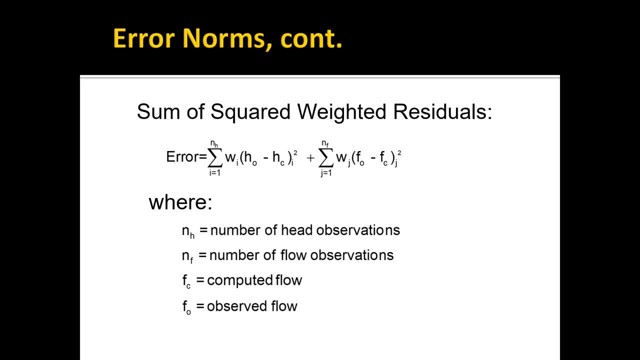 happen here is that both sides of this equation are significant enough or weighted enough that they that they have an impact. so you wouldn't want the left side to be a huge number, on the right side to be a tiny number. you want them to have somewhat of a comparable weight, and so if you follow those guidelines in GMS, 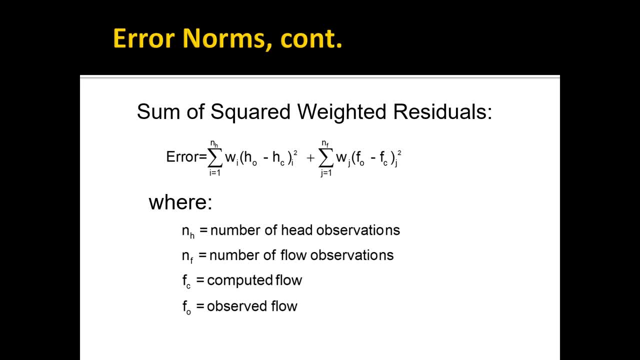 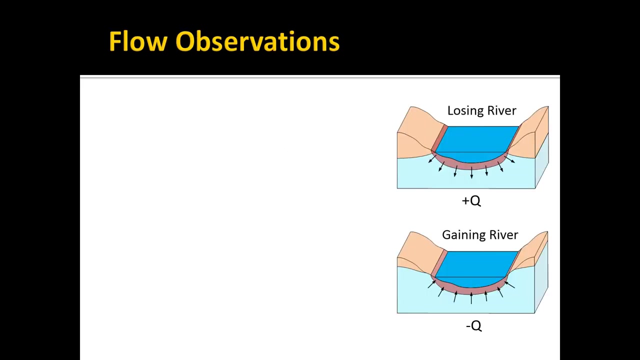 enter an interval calibration target- you know a few meters- and then make your weight, your interval for the flows, about five to ten percent of the observed flow rate. It generally ends up working really well and we'll revisit that when we do our exercises together in class. now coming back to flow observations, some really 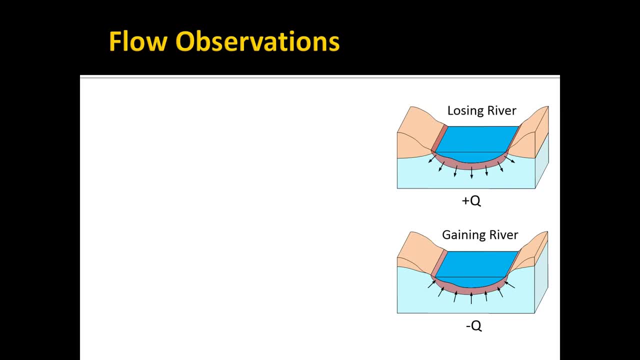 important things to discuss. remember, a river can be a gaining river or losing river and, by the way, we've been talking about gains or losses and strains, but this could be gains or losses and losses or whatever, and that is an aspect of flow on the river. 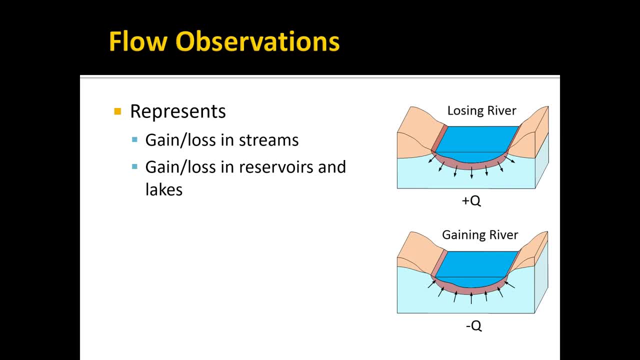 So here's another thing that I like to see, and that is a very important thing to mention here, is when you're dealing with reservoirs and lakes as well. when you're dealing with reservoirs and lakes, you have to factor in evaporation, account for that, and then you have to look at you know how a water 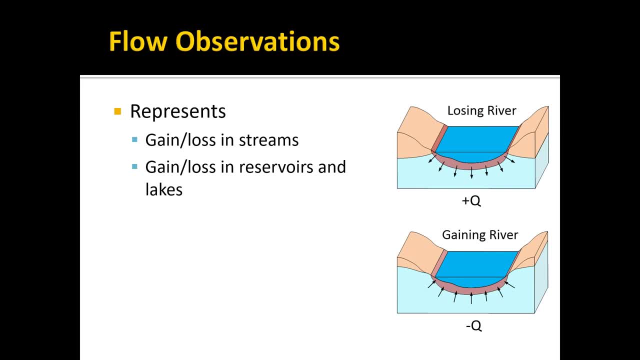 balance- how much is coming into the reservoir and how much is going out- but it's it's possible to get an estimate as to how much water is leaking from the reservoir into the lake or the other way around. People calibrate groundwater models only using head observations, and if you do that without using flow observations in addition to your head observations, it's very likely that your calibration solution- and when I say that I mean the sets of input parameters you use to calibrate your model- may be non-unique. 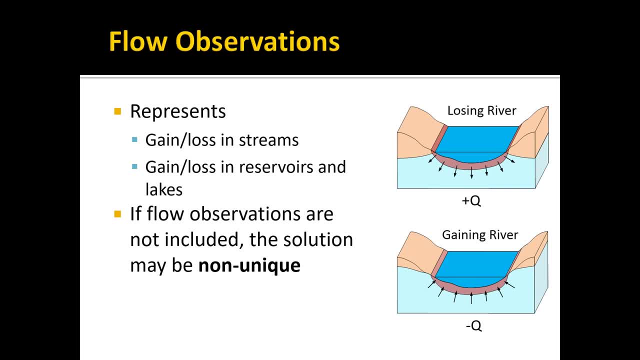 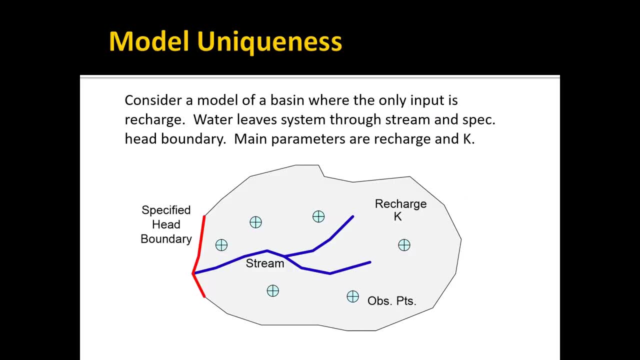 So non-uniqueness is a really important principle when it comes to calibrating models, and so it's something we need to explore in more detail, and in order to explain this, I use this simple model. So consider a basin where the only input to the basin is through recharge, so we have water coming in through recharge and then the water table raises. 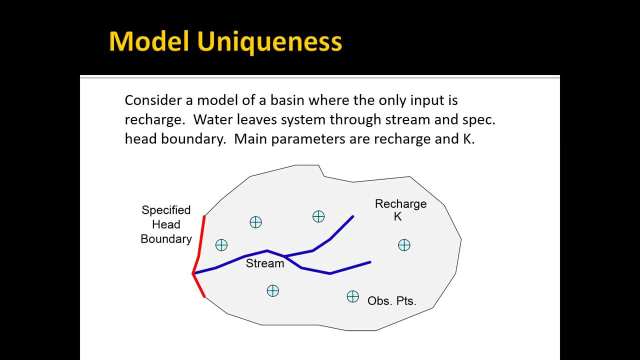 and then, well, it is then discharged to a stream, so we get base flow to the stream. and then maybe on the left hand side, we have a specified head, boundary, a lake or something, and let's assume further that we have some observation wells scattered throughout the 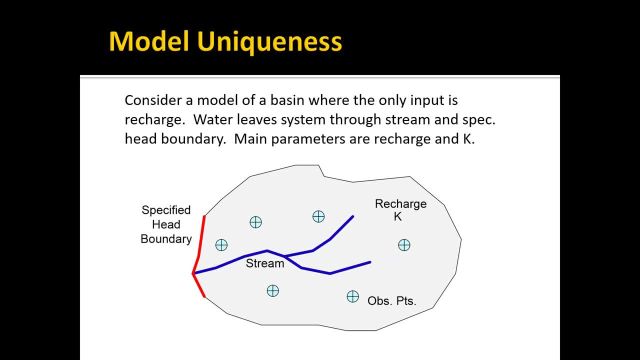 basin that we use to calibrate our model. and in order to calibrate the model, we are going to modify the recharge and hydraulic conductivity parameters, which are the most important parameters. when i say that, i mean when, when you calibrate your model, you'll very quickly discover that the 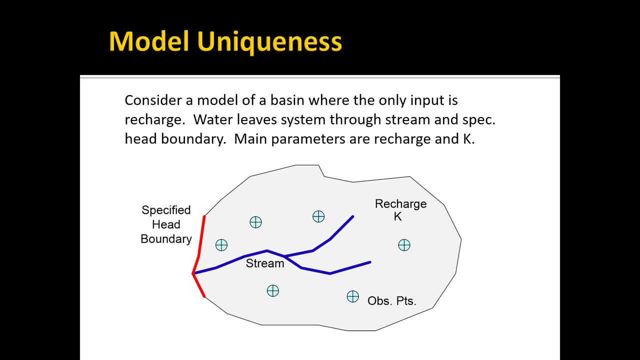 two parameters that the model is most sensitive to are hydraulic conductivity and recharge. you can play with your conductances and some of the other things, but they're only going to have a minor effect relative to these two parameters, and for the purposes of this exercise, we're going to use a little bit more of a different method of modeling the water flow. 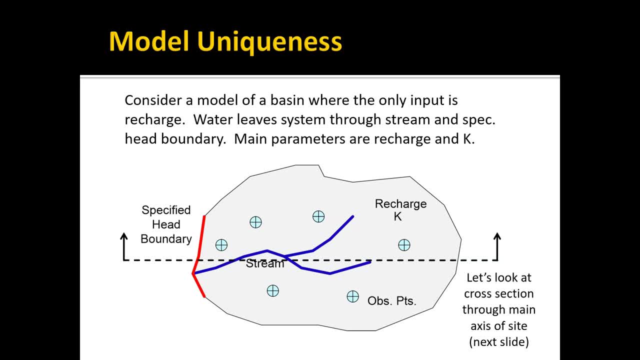 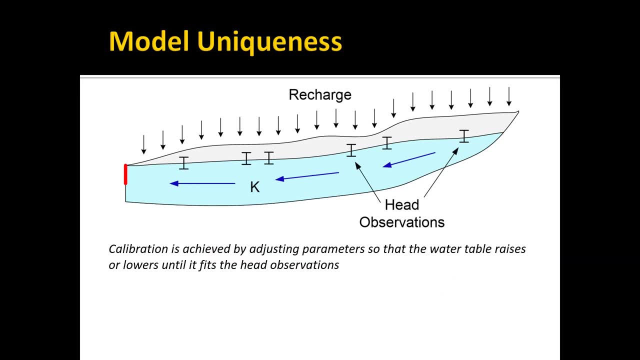 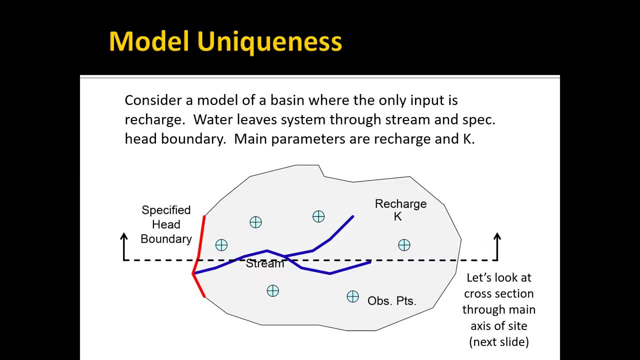 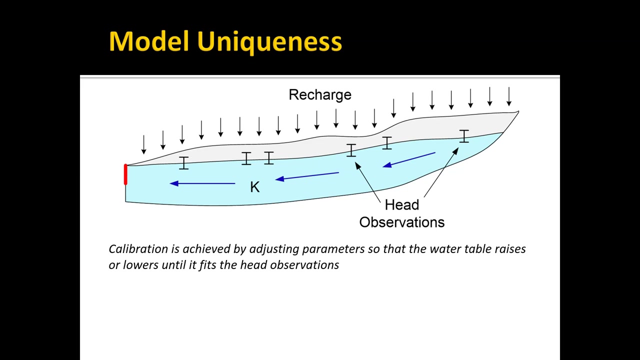 that's what we're going to focus on. so now let's look at cross-section through our model as shown here, and so we're now looking at this slice. so, again, this is along this dashed line, and so these little I shaped symbols on the diagram represent, are the, the elevation of our observed heads, and I've drawn them as a. 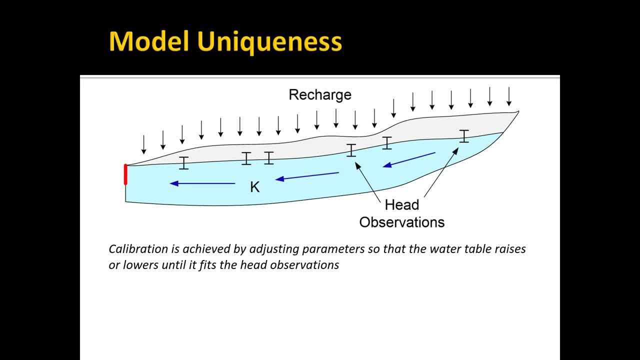 as a target, meaning we just want to get the head somewhere inside that range. so instead of a single value we've got a range that we're trying to move it into. so our objective is to adjust the hydraulic conductivity in the recharge until that water table fluctuates up or down until it matches. 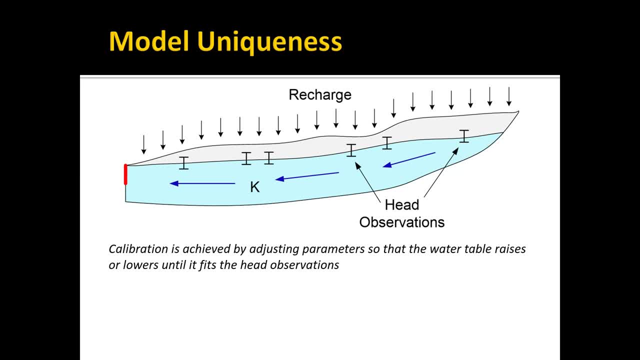 the lift range. so we're looking at that from the perspective of our, our point of view, those head observations. now to start, we're just going to look at head observations. so if, if we look at this model and the water table is too high, if we need to lower the water table, we have two. 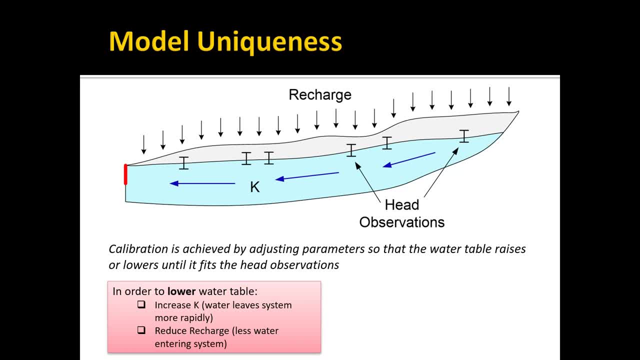 things we can do. we can. we can increase the hydraulic conductivity that causes the water to leave the system more rapidly. you get a flatter water table with a high value of hydraulic conductivity. it doesn't take much head loss as you go through that. so imagine if you had a gravel. 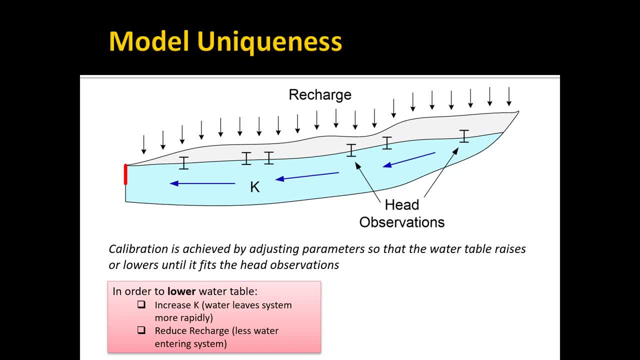 aquifer. it's going to be kind of like a big bathtub and the water table is going to be flat. but if you have a lower permeability aquifer, you know you get a much greater slope because that it mounds. the water table goes up, is it? it has to build up head to push through the low permeability. 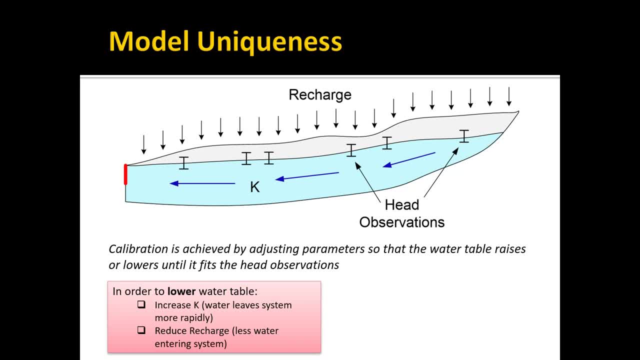 material. another way to do this is to use a water table, and you can see that the water table is going to be a little bit lower than the water table. it's going to be a little bit lower than the water table. so the way to lower the water table is to reduce your recharge if you have less water. 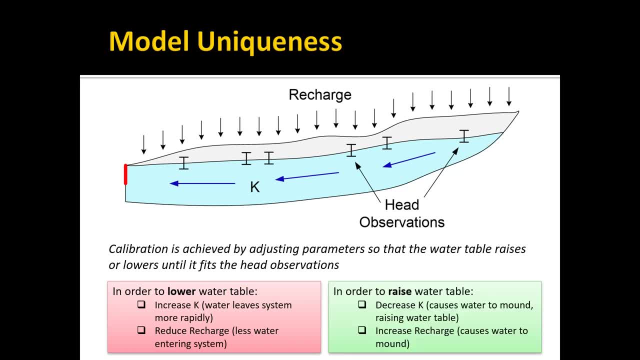 entering the system, you're going to have a lower water table. that should be fairly intuitive now. on the other hand, if we want to raise the water table, we can lower the hydraulic conductivity. it's just the inverse of what we just talked about. or we can increase recharge. both of those will cause the 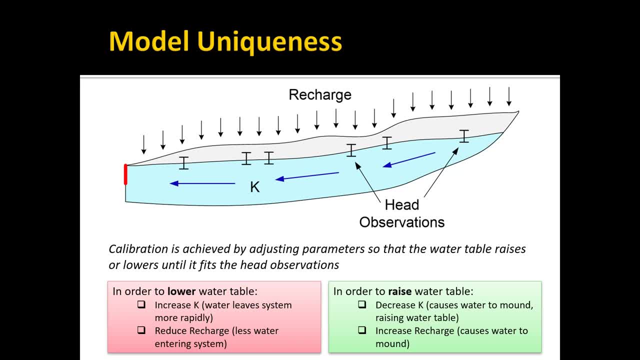 water table. to rise the the water levels, the water will mound in your aquifer and so again to lower the water table. you can either or to both lower or raise the water table. you have both hydraulic conductivity and recharge which independently can can move that up or down, and so 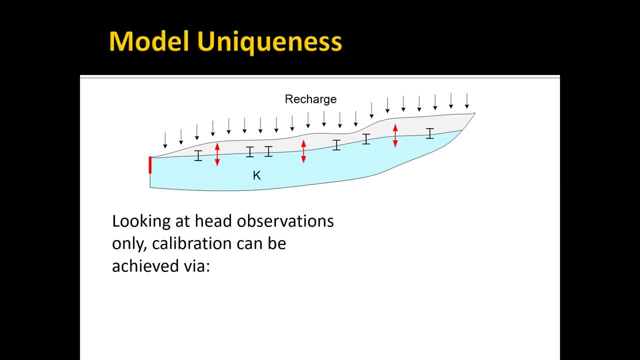 looking at head observations only, if you think about it, we can calibrate the model with a with a low K and low recharge. so, if you think about it, we can calibrate the model with a with a low K and low recharge or a high K and a high recharge. So in other words, theoretically there are 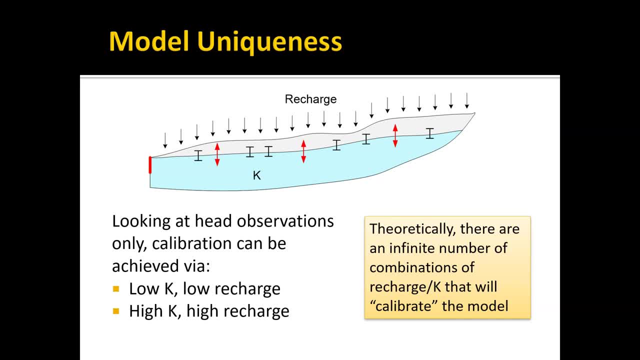 an infinite number of combinations of recharge and hydraulic conductivity that will calibrate them all. Both of them, either one of these independently, will cause the water table to go up or down, And so, yeah, mathematically there is an infinite number of combinations. 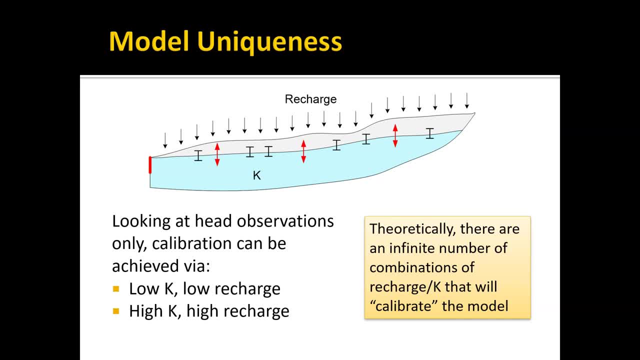 of K and recharge. that will result in a calibrated model. So that's a problem. When we finish calibrating our model, we want to have some assurance that it represents a reasonable representation of what the actual aquifer properties are. Otherwise it's not. 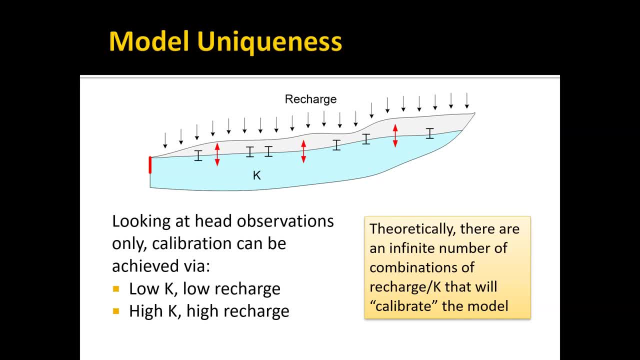 going to be very useful as a predictive tool Because, even though we have the water levels right, the flow rates, the velocity at which the water is flowing, the velocity at which the water is flowing, the flow rates, the velocity at which the water is flowing, the 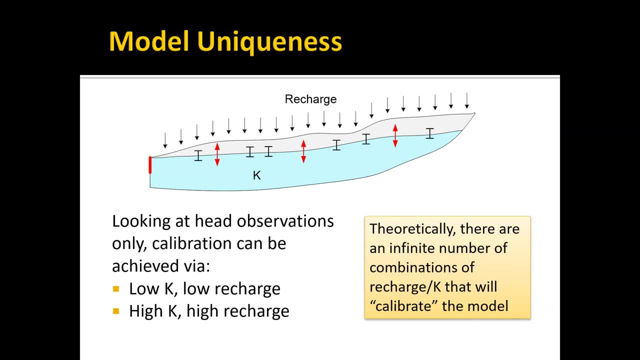 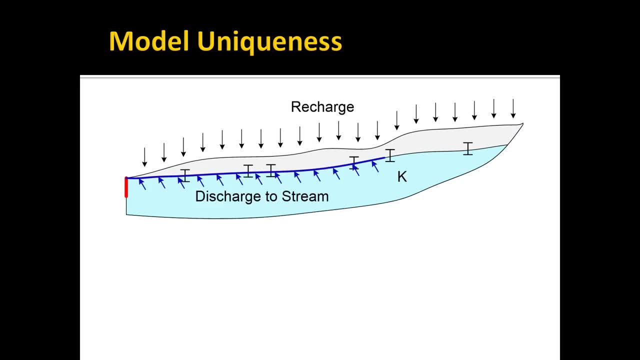 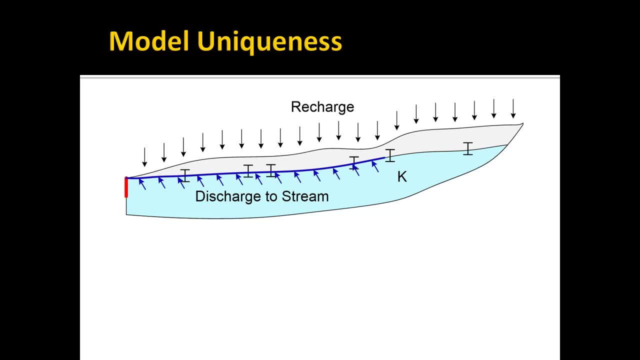 the aquifer is fed completely by gains from the aquifer. It's a gaining stream and the base flow comes 100% from the aquifer. So if we were to measure the discharge at the stream and include that as one of our observations, then basically what that? 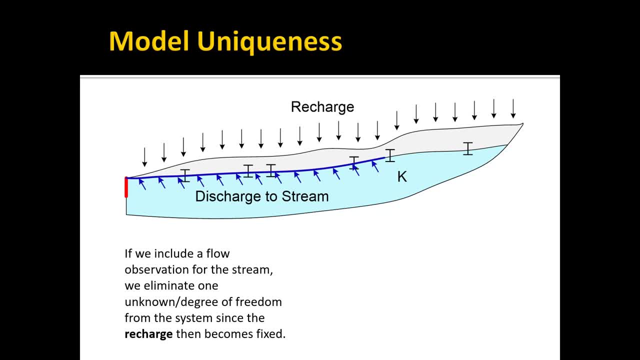 does is that pins down the recharge, because that discharge to the script stream is going to be 100% sensitive to that recharge. if the only input is recharge and the only output is discharge, the stream they're, they're going to be completely tied together. well, there's, there's some discharge to 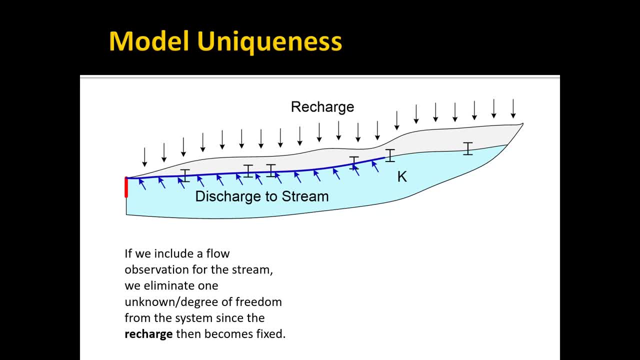 the constant head boundary, but there's going to be a really high level of sensitivity in that, and so by adding a flow observation and changing the recharge until that matches, we've basically eliminated one degree of freedom. so before we had, you know, too many degrees of freedom, and it's kind of 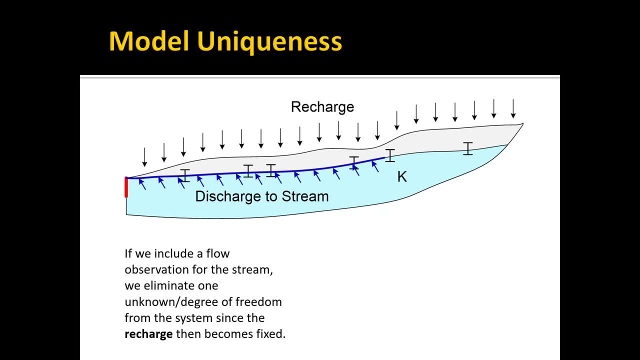 like having you know more, more equations, and we have unknowns. well, this, get this gives us a balance that we can solve for. you know more, more equations, and we have unknowns. well, this, get this gives us a balance that we can solve for, and at this point, the only remaining unknown is a hydraulic conductivity, and 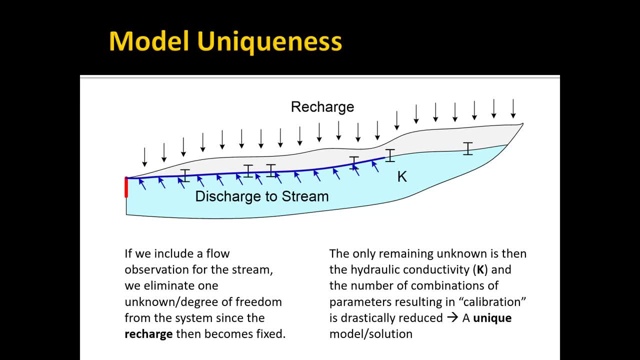 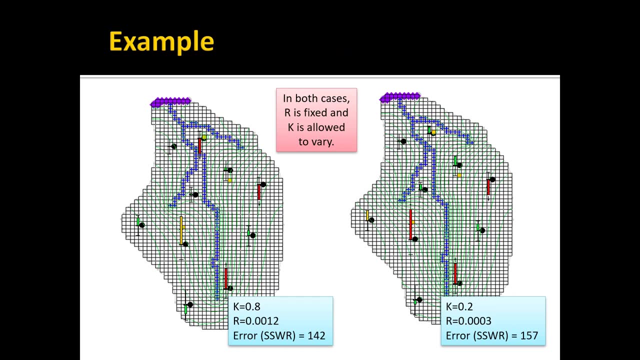 the number of combinations of parameters that will calibrate the model is drastically reduced, so we have a more unique model or solution to our calibration process. so to illustrate this, I did a little experiment and on the left we have- this is a model that we're going to be using in class and it's very similar to 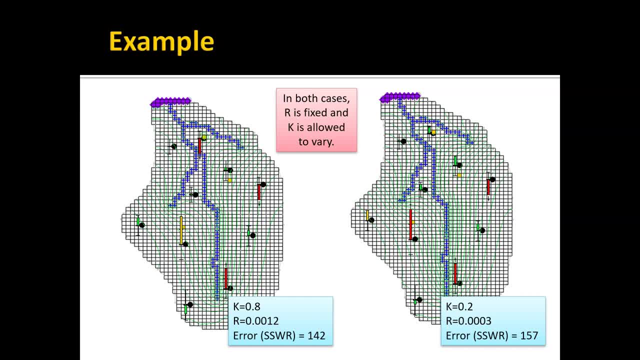 the one I just showed you. it's a. it's a closed basin. at the very northern outlet there's a constant head boundary condition. it has a stream in the middle that's completely fed through base flow from the groundwater. we have a number of head observations, and so what I did is I using head observations? only I used a. 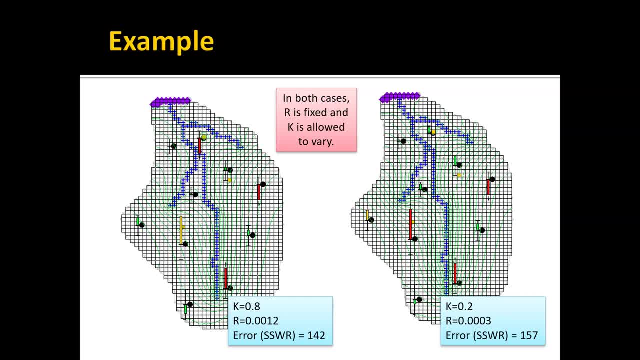 parameter estimation utility. and in the first case I started with, I fixed the recharge to a low amount, point zero, zero, one, two, and then I solved for the hydraulic conductivity that that gave it a low error and the sum of the squared weighted residuals at the end of this process was 142. now keep in mind that it. 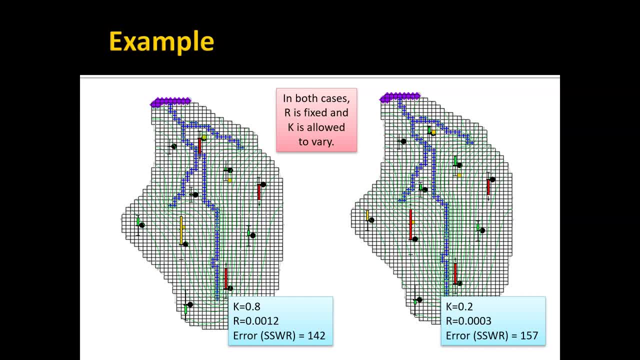 starts out in the thousands, so 142 is a really low number in this case, and so this model was calibrated and if you look at these calibration targets, so the- the green means a really good match, the red means a medium match. yellow or red and yellow is not great, but overall it is. 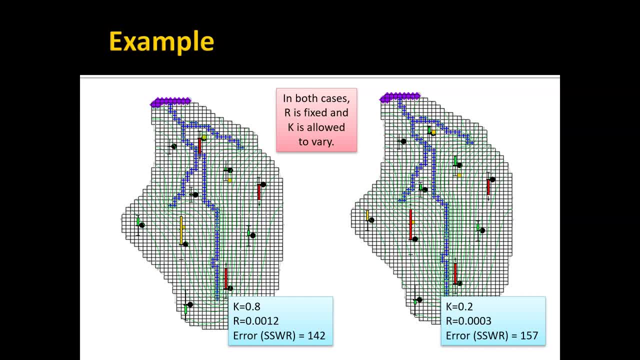 calibrated reasonably well, especially since I'm only using a single value of hydraulic conductivity and recharge. if we spatially vary the hydraulic conductivity and recharge, we could get an even better fit, but but that's. that's a good solution now in this. in the next case I changed. 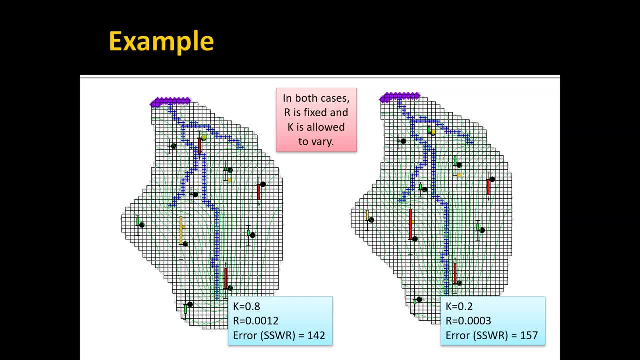 the recharge to point zero zero three, so I changed it by a factor of four, I reduced it by a factor of four and then, using the parameter estimation utility, I optimized that and solved for a value of K and it got it down to 157, which is not. 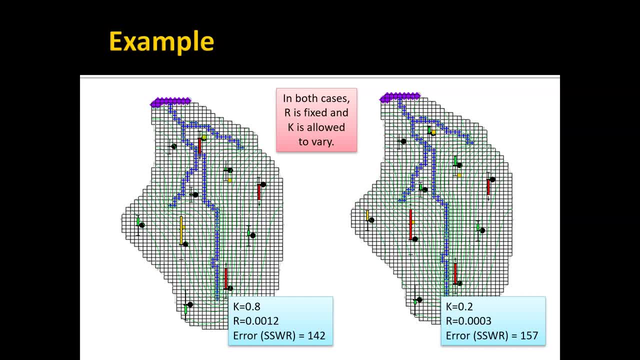 exactly the same, but they're both really close- and that was the point of diminishing returns- and notice that it reduced the hydraulic conductivity to be one-fourth of the value we have on the left. so, in other words, both of these models are calibrated, but they're very different. 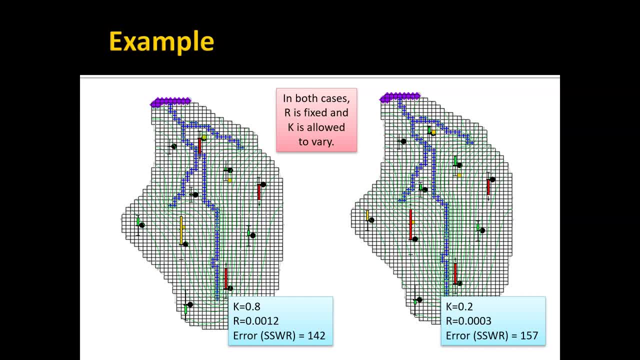 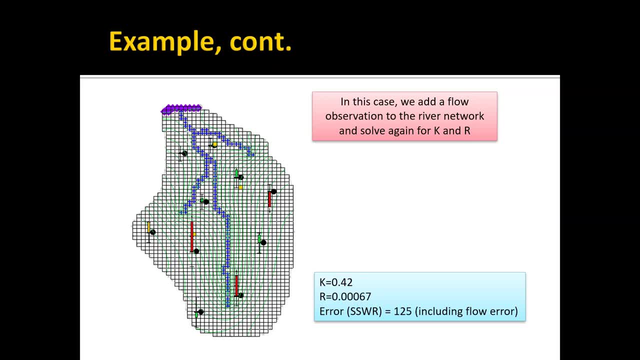 they differ in recharge and hydraulic conductivity by a factor of four. and then, finally, in the last case, I added a flow observation to the river network and I then used the pest utility to solve for both hydraulic conductivity and recharge. in this case, I got the sum of the squared weighted residuals down to 125, and that 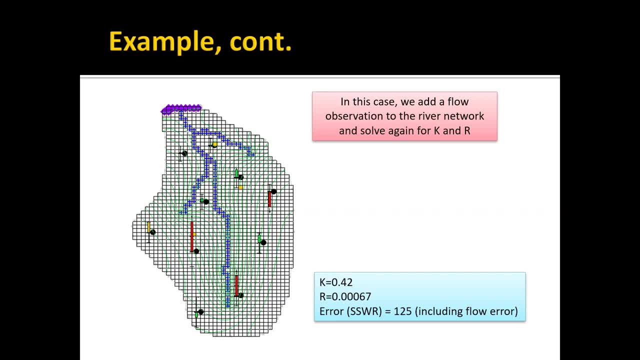 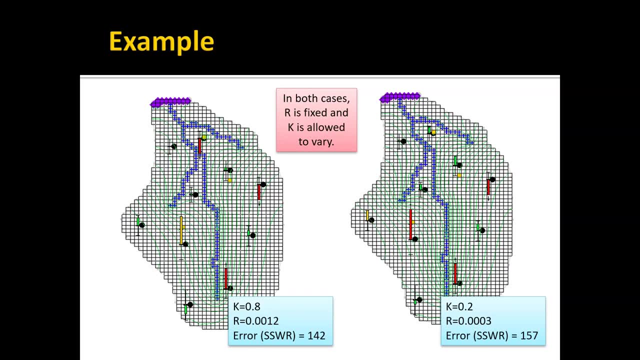 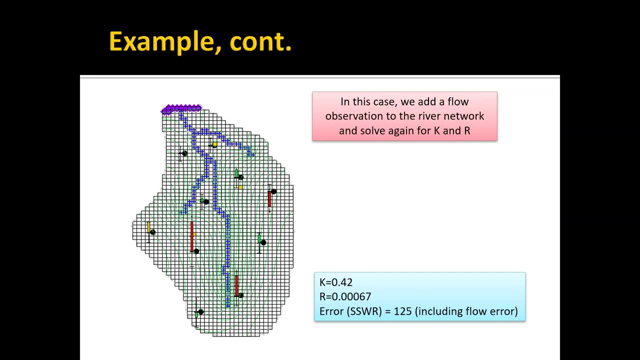 includes the flow error in this case, and I ended up with a K value that was kind of between these two values and a recharge value that was between these two values and resulted in it was also calibrated. so essentially I have three calibrated models, but but this final one I have way. 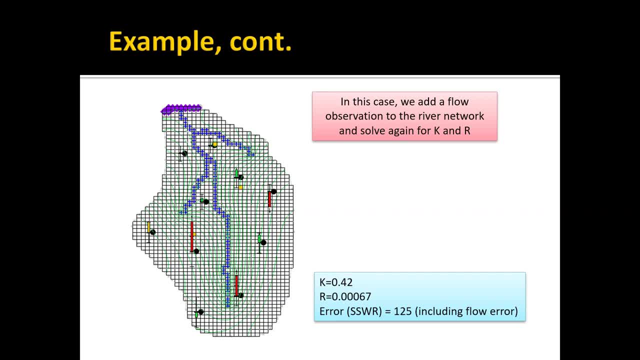 more confidence in because it, by using a flow observation it was able to minimize, it was able to find a solution that I think we can have a lot more confidence in and more confidence that this is a unique solution. now, later, when we talk about the parameter estimation utility, I'm going 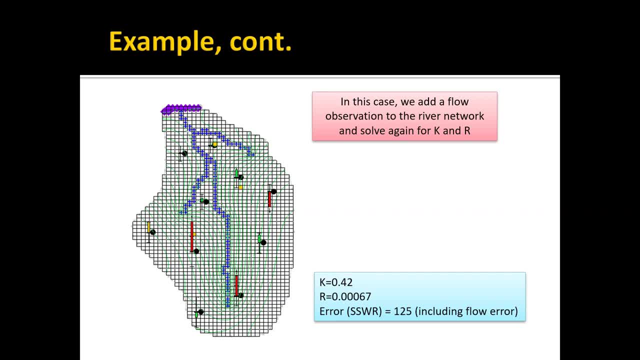 to show you. there's actually a numerical measure we can use to determine, to get an idea whether a model is the level of uniqueness to the model, and we'll talk about that later. but the point is, if you don't have a flow observation, you need to really worry about whether or not you have a unique, unique or a non unique. 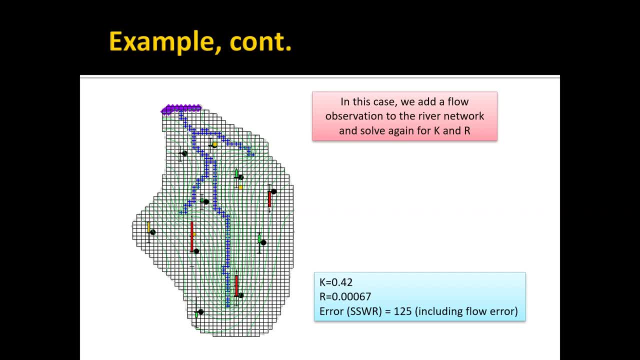 model and something that we always need to be aware of when we're doing model calibration, and for that reason we generally have to have. we either have to have a flow observation or we have to just guess at what the stream flow discharge would be. to pin it down, sometimes you have to make educated